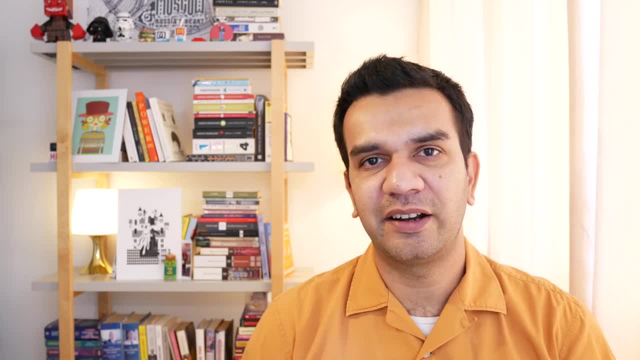 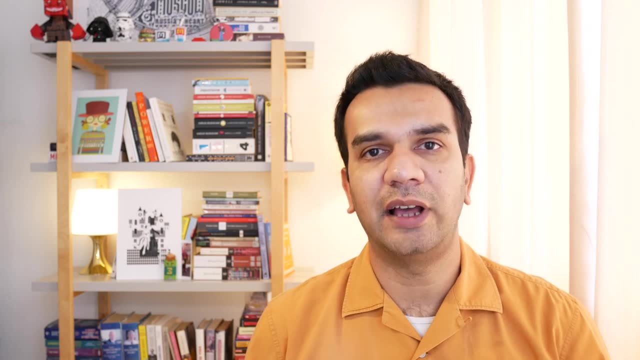 put it very simply, it's called numeric distribution. So while numeric distribution is extremely simple to understand, real life is not always that simple. Imagine a situation where you have distribution in a large number of stores, but all of these stores were actually small stores and therefore their total 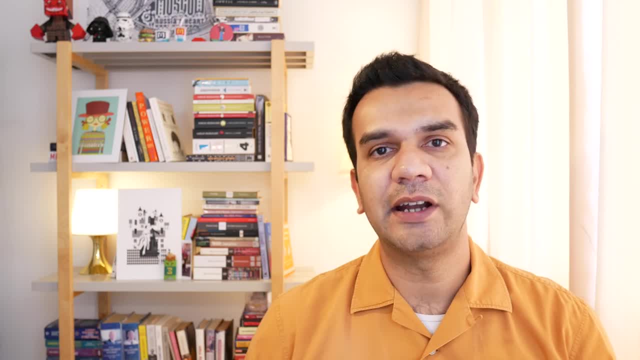 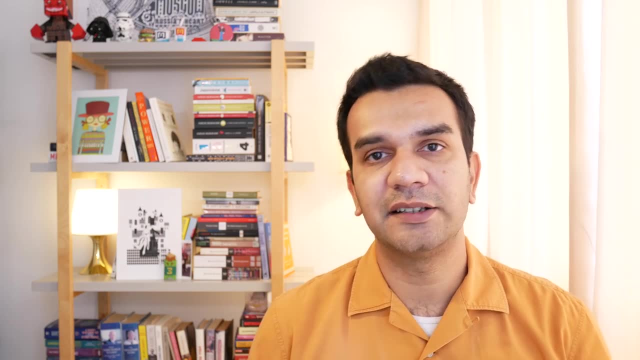 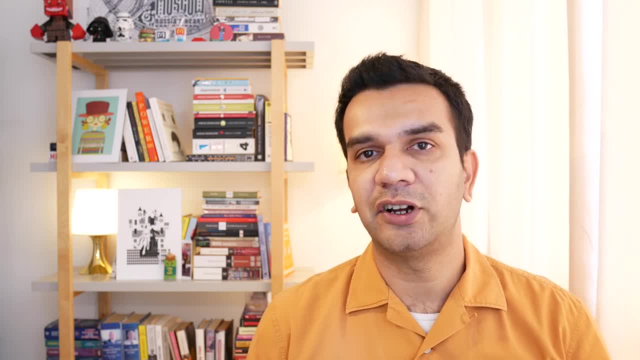 Your power of distribution or the number of customers that you have in that region is going to change. Your power of distribution or the number of customers that you have in that region is going to change, which seems pretty high, might actually not be that strong and, as a result, your sales would be low. 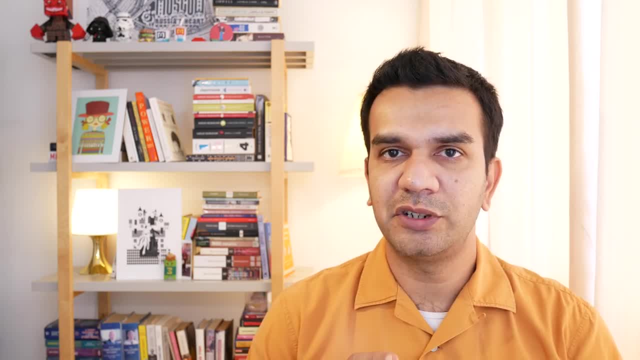 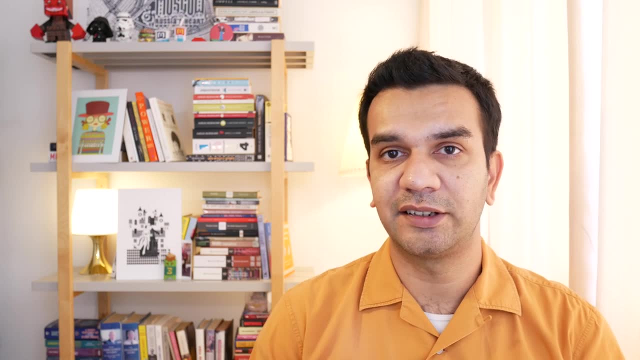 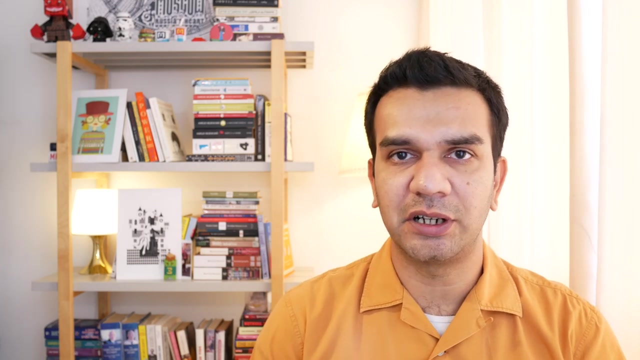 therefore, let's start getting into the next concept around distribution, where the size of the store plays a role. what this means is, if a store has higher total sales, it matters more than a store which has lower total sales. and that is where the next measure- acv- all commodity value. 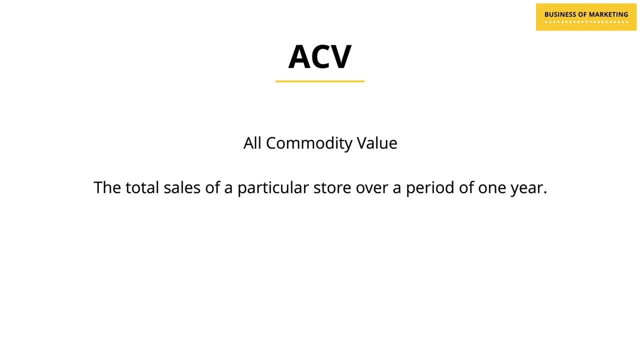 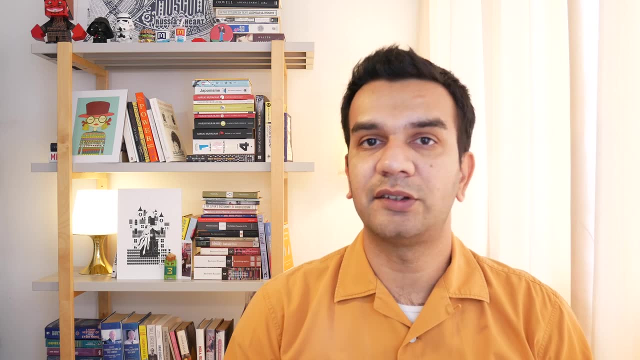 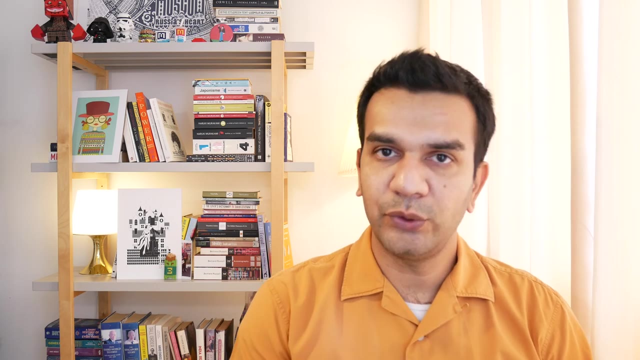 comes in acv or all commodity value is simply the total sales of a store over a period of one year, because acv tells you the total sales of a store. imagine a situation where you knew the total sales of all the stores in a particular region, so using this, you would be able to find out which are the 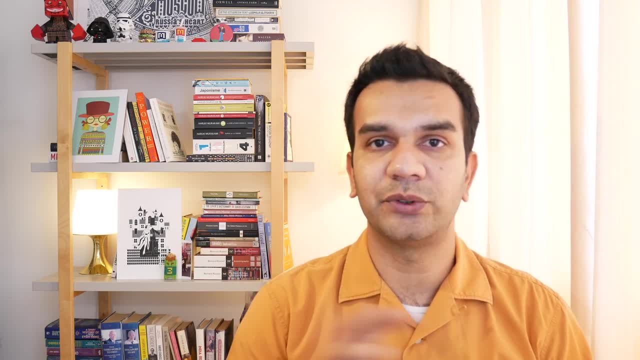 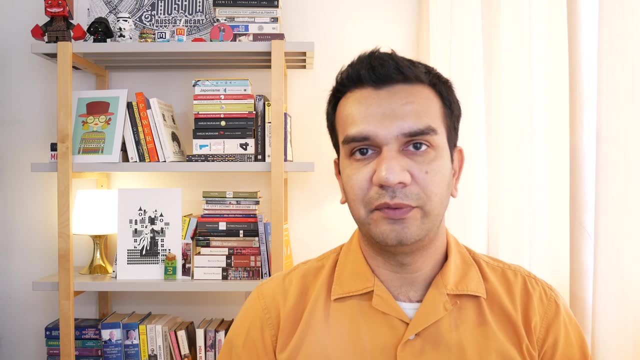 most important stores and which are the least important stores, which is stores with the highest sales, as well as the stores with lower sales. and that brings me to the next important measure in distribution, which is percentage acv. it is also called percentage acv distribution and also 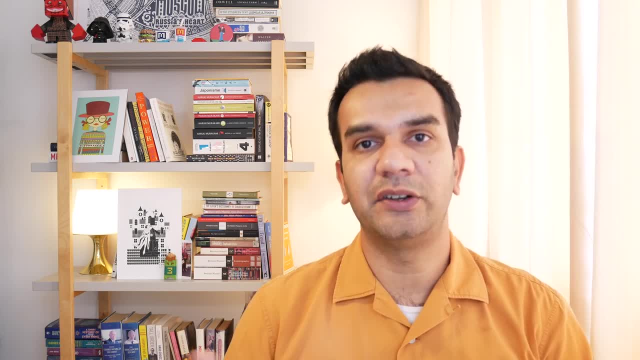 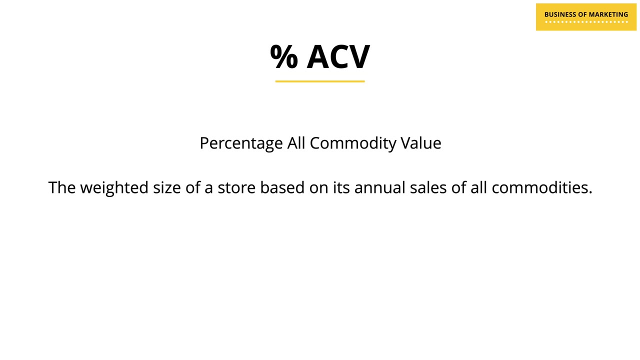 sometimes referred to as percentage acv, weighted distribution. you can call it whatever you want. for simplicity's sake, i will refer to it as percentage acv in this video. percentage acv is simply the weighted size of a store based on its annual sales for all commodities. let's try and 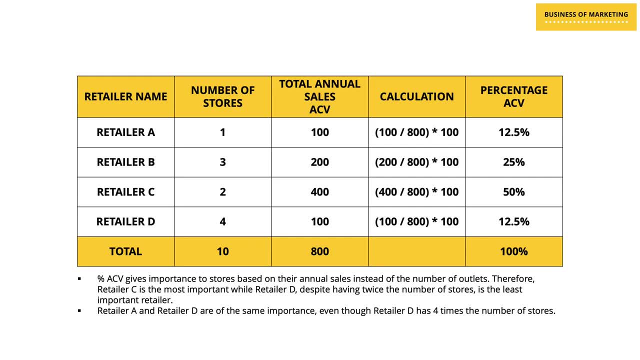 understand this with the help of an example. so imagine there are four retailers- a, b, c and d- with one, three, two and four number of stores, which is total. there are 10 stores in that region and their respective annual sales value, or acv, was 100, 200, 400 and 100 respectively. so the total acv for that region would be 800. using this, we 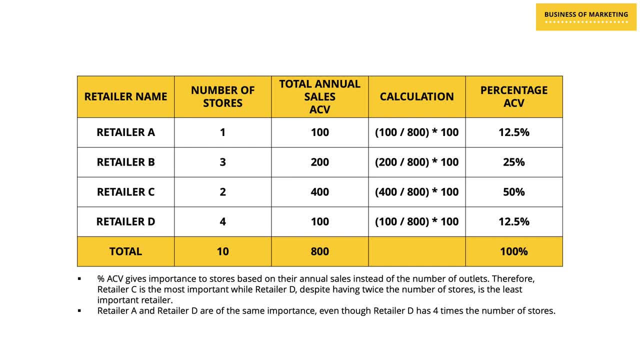 can find out the percentage acv of all the stores. when you divide the acv of a single store or a single retailer by the total acv for that region region and multiply that by 100, you get the percentage ACV. In this case it works out to be 12.5% for retailer A, 25%, 50% and 12.5% for the remaining. 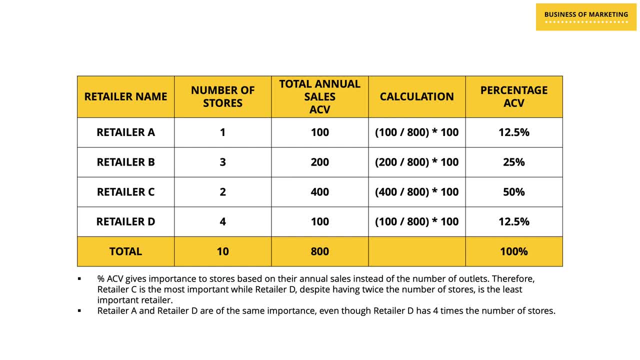 three retailers. Percentage ACV actually gives importance to stores based on their annual sales instead of the number of outlets that they might have. Therefore, retailer C is the most important retailer, where the percentage ACV is 50%, while retailer D, despite having twice the number of stores, is the least important retailer. 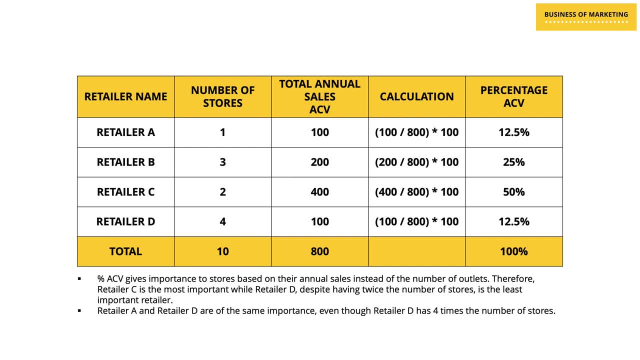 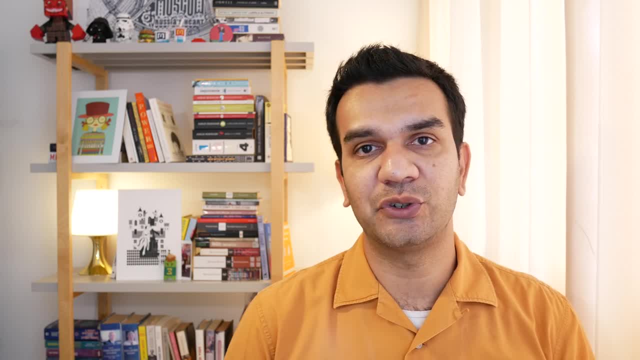 Retailer A and retailer D are of the same importance, even though retailer D has four times the number of stores. So you might ask: what does this have to do with my distribution? Let's look back at the same example to try and understand this a little better. 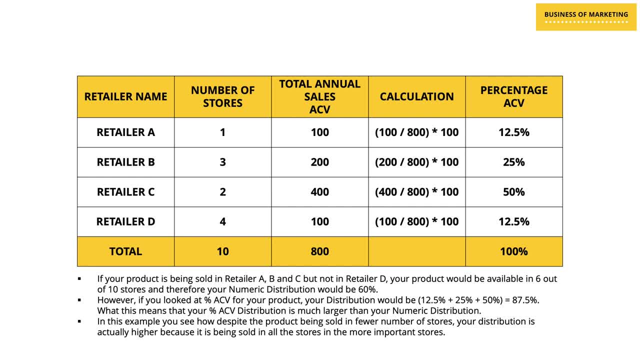 If your product is being sold by retailer A, B and C, but not by retailer D, your product would be available in 6 out of 10 stores And therefore your numeric distribution should be 60%. However, if you looked at percentage ACV for your product, your distribution would be 12.5%. 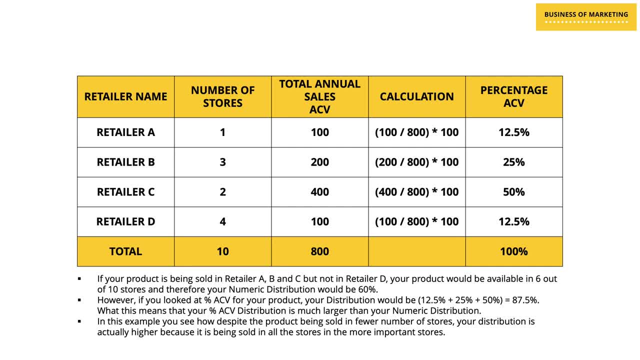 plus 25%, plus 50%, which is 87.5%. What this means is that the percentage ACV distribution is much larger than your numeric distribution. So in this example you see how, despite the product being sold in a fewer number of stores, 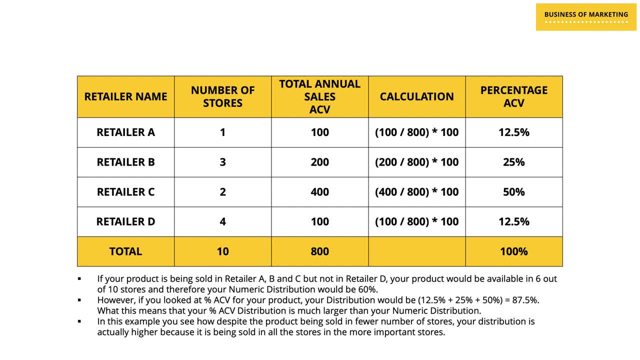 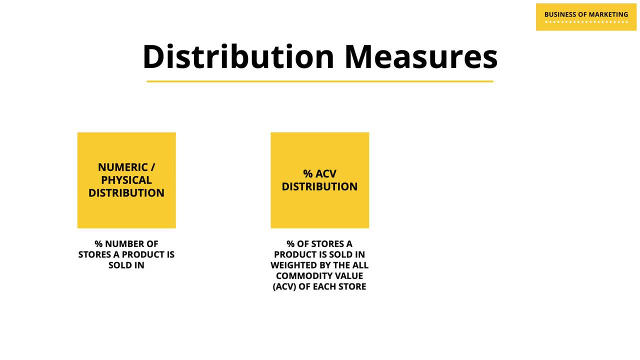 your distribution is actually higher Because it is being sold in all the stores, or all the more important stores. So we have seen two important measures of distribution, The first one being numeric distribution or physical distribution, which is simply the percentage number of stores a product is sold in. 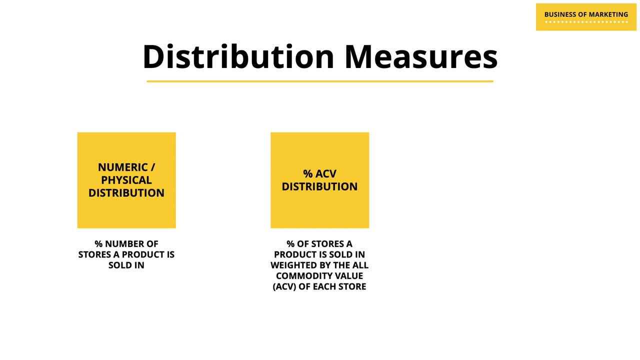 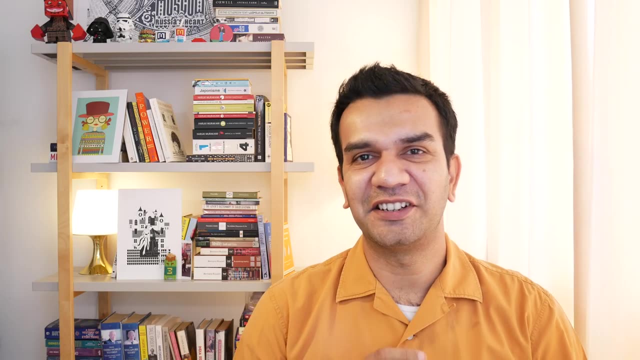 The next one that we spoke about is percentage ACV distribution, which is the percentage of stores a product is sold in, weighted by all commodity value of each store. Now, let me add another small complication to this conversation. Now what if your product is something which belongs to a category where it doesn't really? 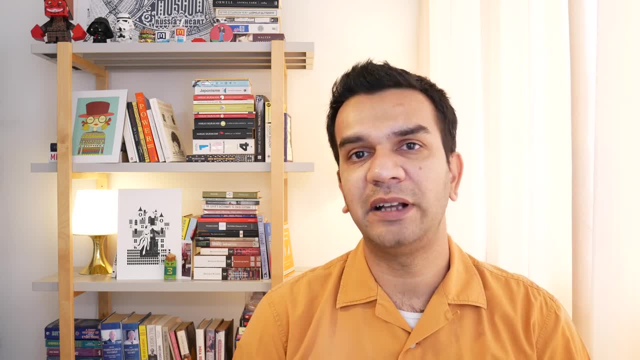 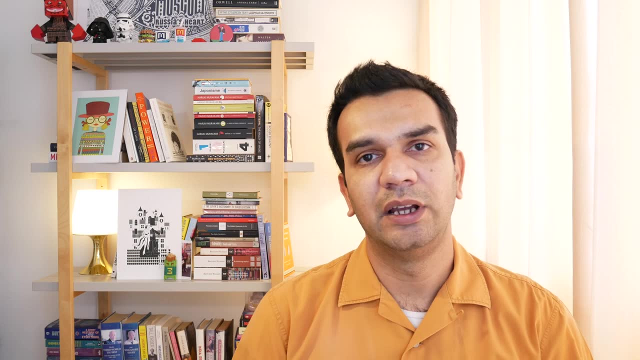 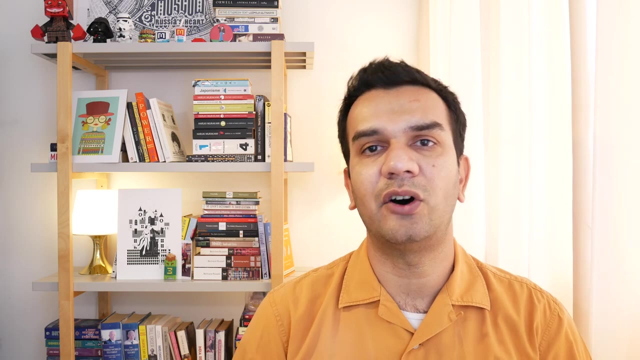 matter how big the size of the store or how big the ACV of the store actually is. For example, your product is some environmentally conscious brand of shampoo. It appeals to people of a certain type, who are also the same people who shop for similar organic or environmentally conscious products. 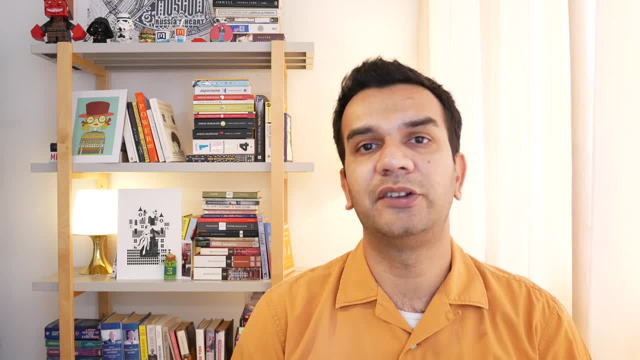 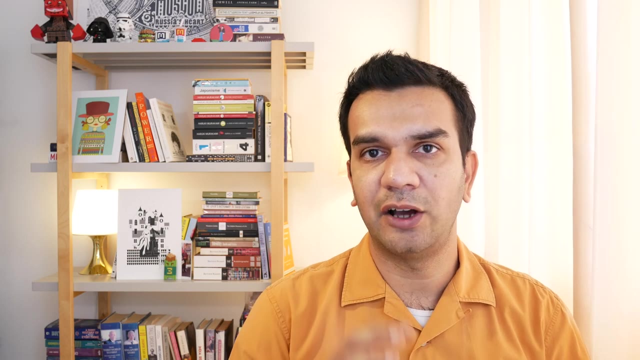 And these people tend to frequent stores which are into selling of these environmentally conscious and sustainably created products. In such a situation, what is more important than the size of the store is the size of the category in which your product operates. In this case, it is environmentally conscious products. 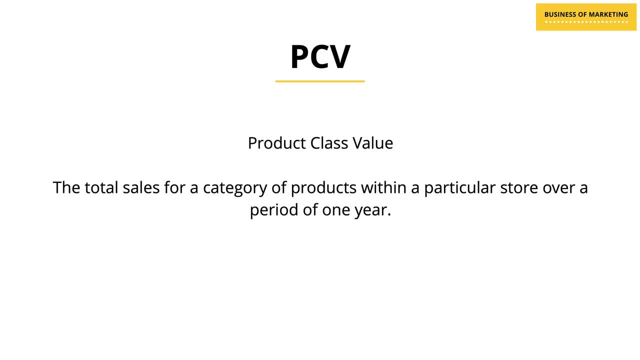 And this is where the next measure of distribution comes into play, Which is product class value or PCV. Unlike the ACV, which is the total sales of all products in a store, the PCV is the total sales of a particular category of products within a store in one year. 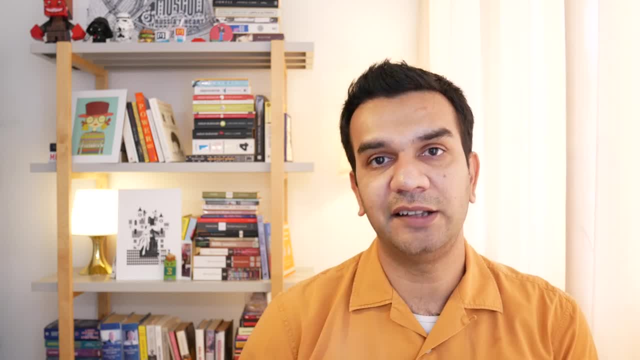 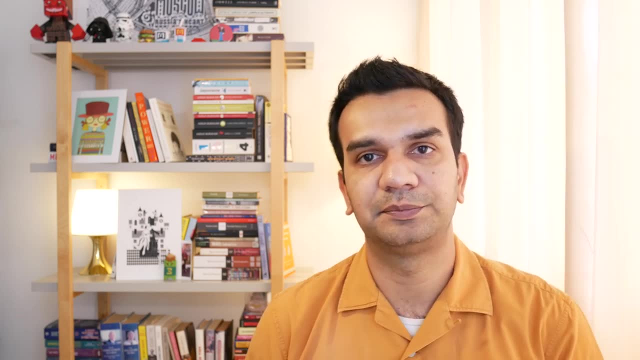 And basically what this means is that the stores where the sales for your category is higher would be more important to you than stores where the sales of your category is lower. And that brings me to the next important concept in distribution, which is percentage, PCV or. 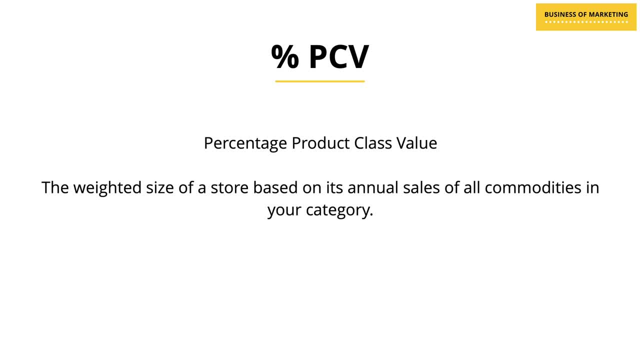 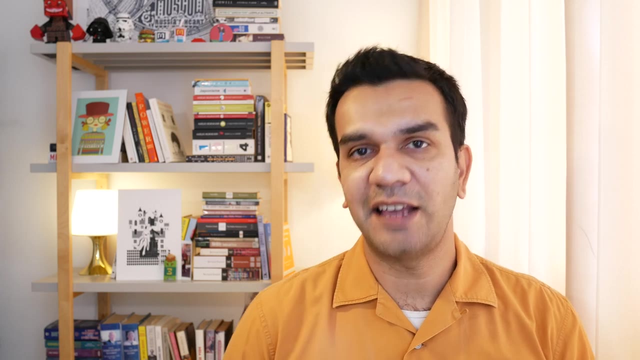 percentage. product class value. It is simply the weighted size of a store based on the annual sales of all commodities in your category or a particular category. So again you might ask: what does this have to do with the distribution of my product? Let's look back at the same example with some changes to try and understand this a little. 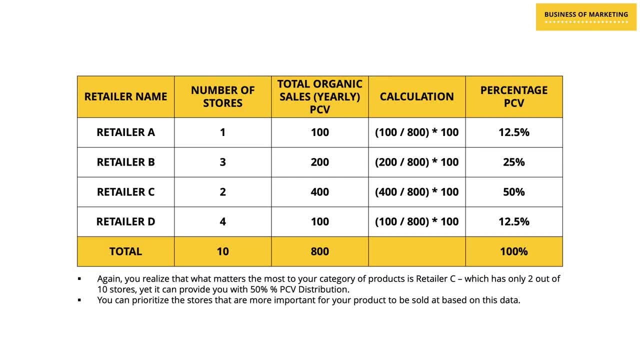 better To keep it simple to understand. I have simply changed ACV to PCV in column number 3.. Over here you can realize that what I have done is that I have simply changed the distribution of my product. So what matters the most to your category of products is retailer C, which has only 2.